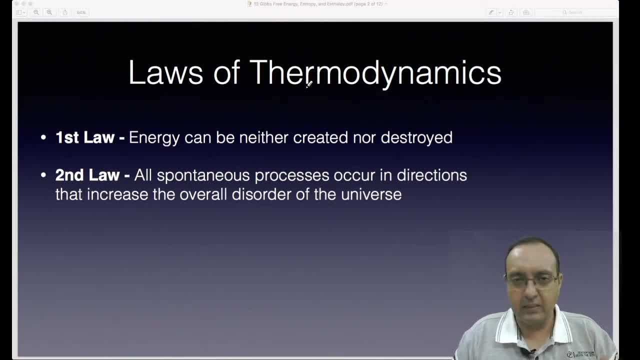 with the formulations of the laws of thermodynamics. There are actually four laws of thermodynamics, but for living systems only two are of our concern. The first law states that the energy can neither be created or destroyed, So it is the law of conservation of energy. So the total 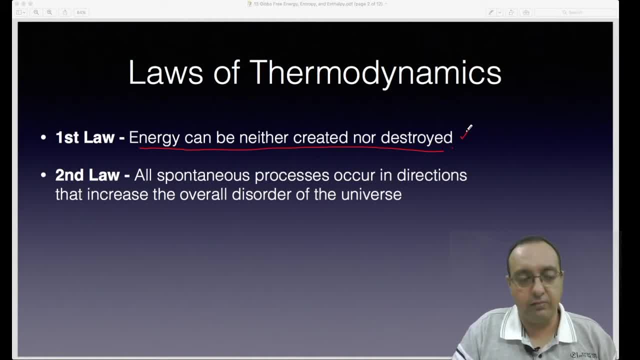 amount of energy in the universe is constant. So that's the first law. It's also known as the law of conservation of energy. The second law states that all spontaneous processes. spontaneous means we don't have to provide energy to them for them to occur. All spontaneous processes occur in 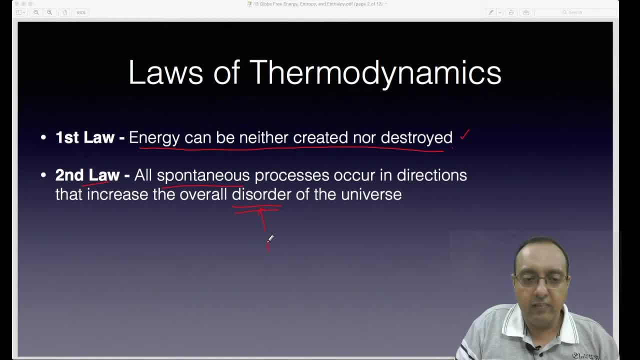 the universe- This is the key term here- disorder, and that relates to the term which is the entropy. Now, the laws of thermodynamics were actually formulated in the industrial revolution, when there were a lot of developments around steam engine and development of machines that could. 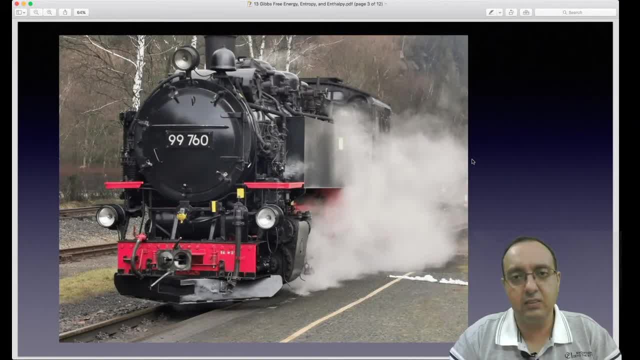 automate human work. So, for example, steam engines. they operate on the principle of temperature differences. So there is a place where there is a temperature difference between the temperature is a high temperature. there is a place where there is low temperature and transfer of that energy drives work. but that's not how living organisms work. if 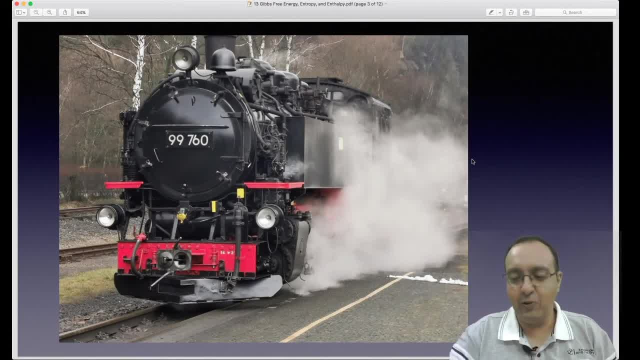 you have noticed, we are not steam engines and we don't operate at such extremes of temperature. we operate at a fairly constant temperature and if you look at ecology or the, for example, exchange of nutrients in the environment, you will see a cycle which is also sometimes called a food chain. so this 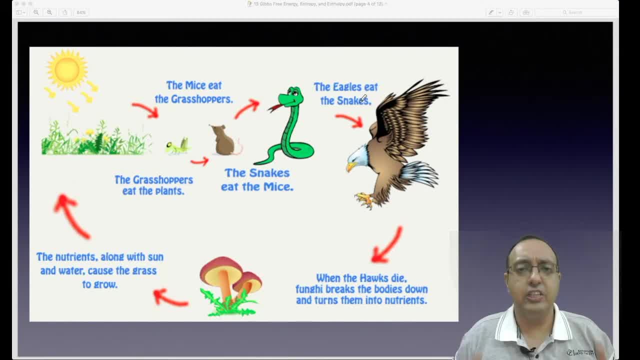 food chain is very easy to understand. all of our energy in our biosphere basically comes from the Sun. okay, so Sun is the ultimate source of energy. the solar energy is used by plants, although there are some organisms which can use inorganic nutrients, for example nitrifying bacteria and other chemo. 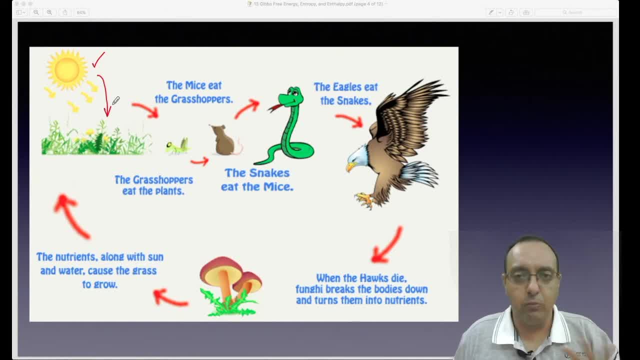 autotrophic bacteria, but those are the exceptions, most of the organisms. they start their food chains here. the solar energy is taken up by the plants to make up their biomass, which is eaten by other small animals, for example herbivores, grasshoppers, and then those 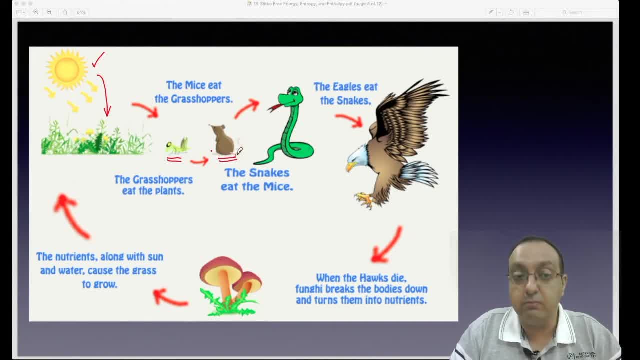 animals are eaten by carnivores, such as mouse and other larger carnivores, and then omnivores, for example humans. and when these organisms die, for example carnivores, omnivores or even herbivores, they die, they their bodies and their nutrients present in them. they are 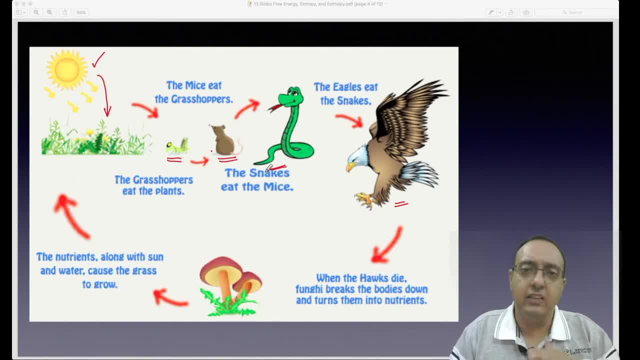 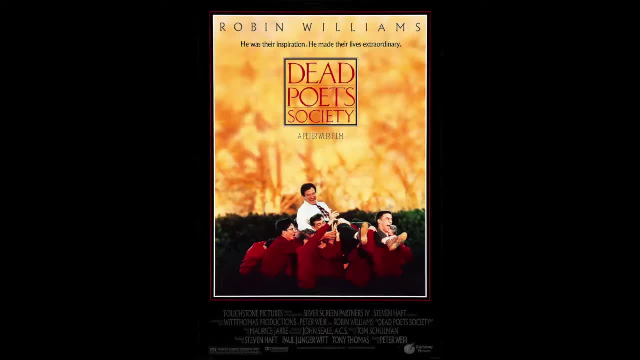 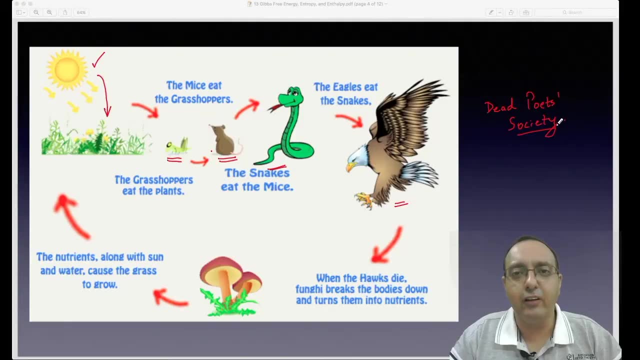 decomposed by bacteria and fungi and they are released back into the environment and that helps the soil grow, right? so if you have watched the movie dead poets society, highly recommend you watch that. it's pretty good movie- dead poet society. we are all fodder or fertilizer for dandelions, right? so 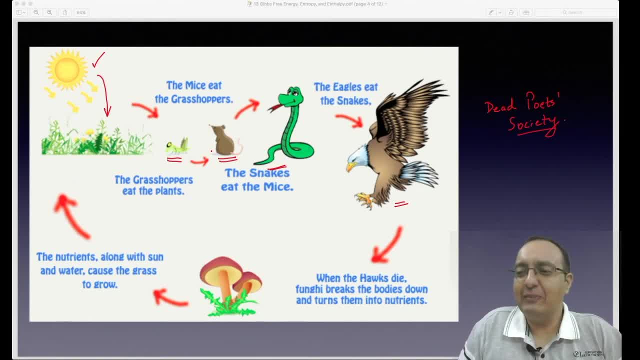 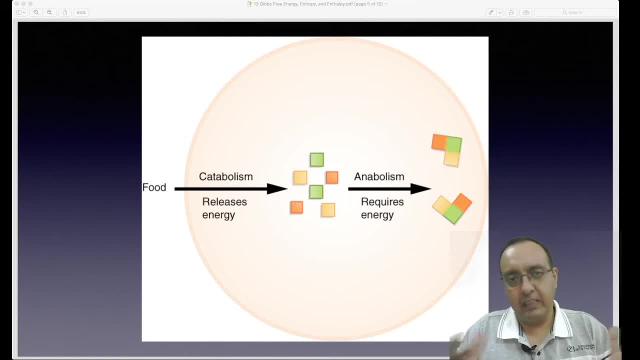 carpe diem. okay, anyways, let's get back to it. so the catabolism and anabolism. I think you are pretty familiar with these terms. catabolism and anabolism basically work around these laws, these laws of thermodynamics, because what happens is: 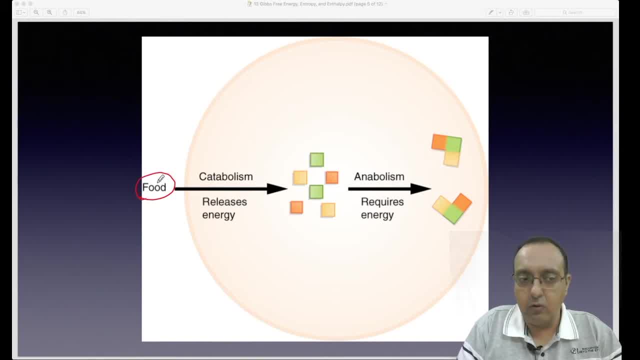 these food molecules, whether they are herbivores or carnivores, are only mors. these food molecules are broken down by catabolic reactions. these f be, for example, your glycolysis, Krebs cycle, pentose, phosphate pathway, beta-oxidation of fatty. 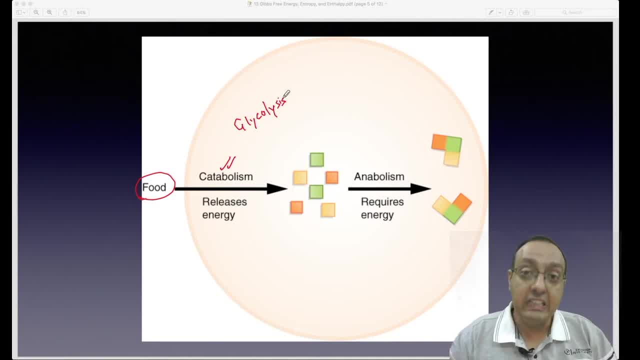 acids. all these nutrients are broken down. They release energy in the form of NADH and FADH2 and some ATP, and this is converted into ATP, finally by electron transport chain or oxidative phosphorylation, And we have the simpler nutrients then available to us. Now these need to be. 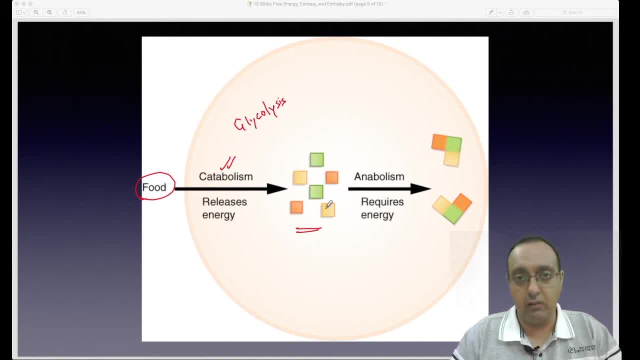 put together to form our tissues, our cells, our biomolecules, DNA, RNA, proteins, etc. Now this requires energy and this is where this energy is used up. So ATP and NADPH: These are the two basic molecules. There are other secondary accessory molecules. 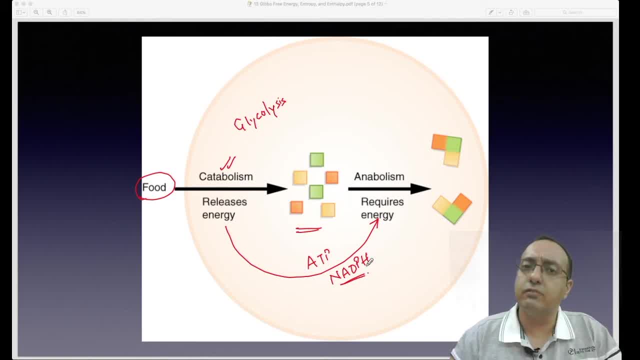 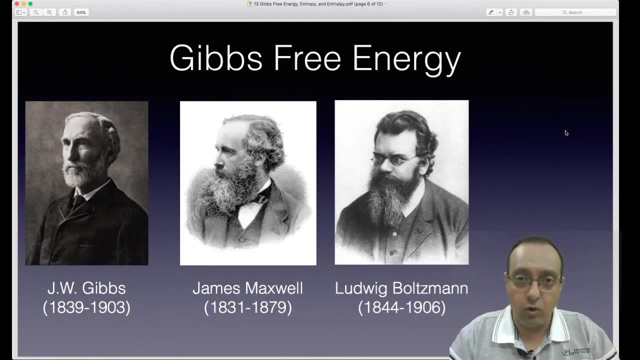 but most of the time these are ATP and NADPH which are driving the anabolism. So the concept of Gibbs free energy. Now let's come back to the thermodynamics and let's talk about Gibbs free energy. Gibbs free energy was basically developed by a professor at Yale University. 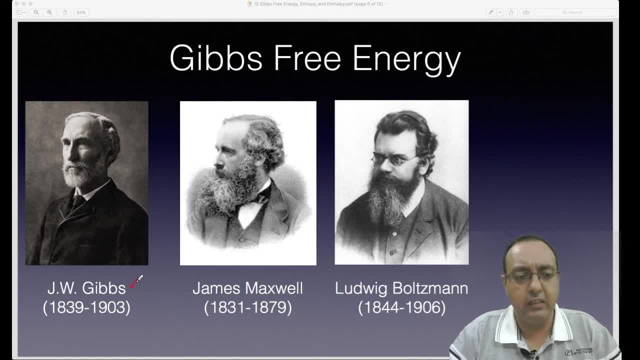 Josiah Willard-Gibbs or Josiah Willard-Gibbs, not sure, And in conjunction with other statistical mechanics scientists, for example James Maxwell and Ludwig Boltzmann, they formulated the basic postulates of Gibbs free energy. So Gibbs free energy was basically developed by a professor at Yale. 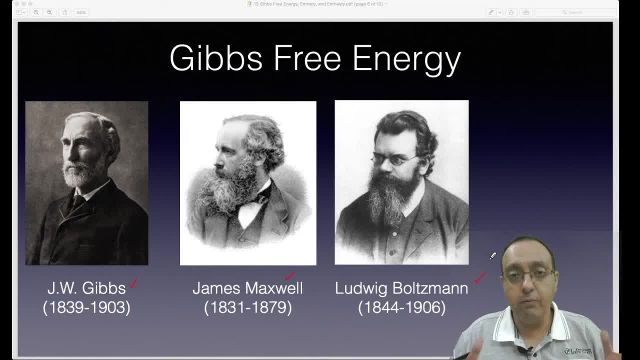 University, Josiah Willard-Gibbs or Josiah Willard-Gibbs, not sure, And in conjunction with other statistical mechanics and thermodynamics. And one of the important components to describe whether a reaction is spontaneous or not, which means whether it can occur or not- is the concept of Gibbs. free energy and the free energy. 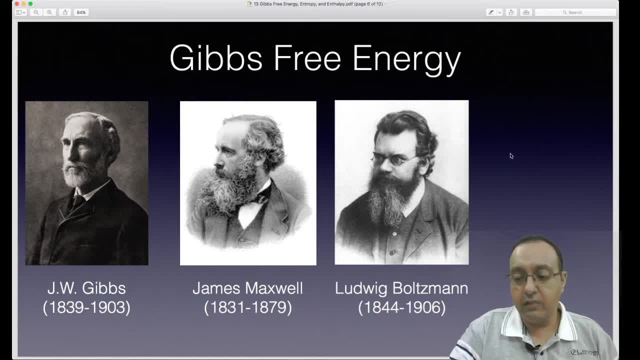 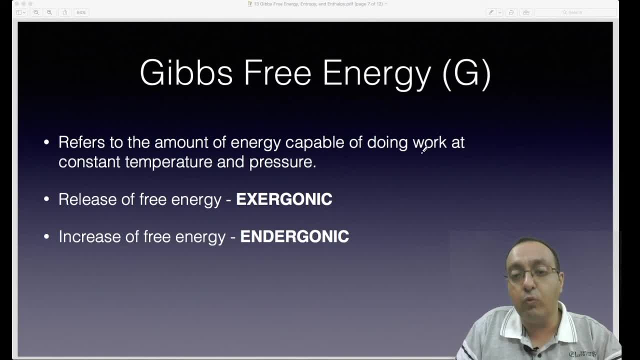 change. So what is it about? Let's see, Let's define our terms. First, what is Gibbs free energy? Gibbs free energy basically refers to the amount of energy capable of doing work. This is the important distinction here. which is capable of doing work? because this 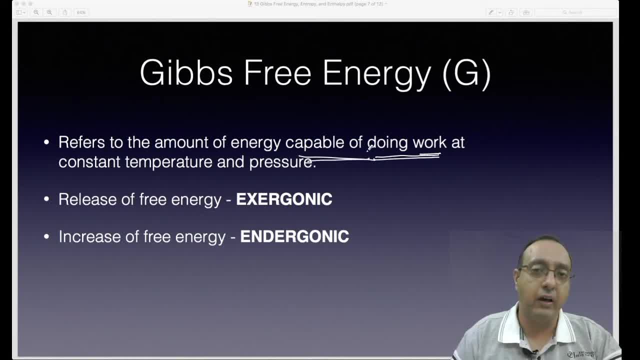 is a heat-free energy And there is a lot of heat which is generated and released by organisms, which is called random heat usually, For example, even like, for example, now I am sitting in my room and I am emitting some heat, which is which can be detected by infrared radiation, but this is 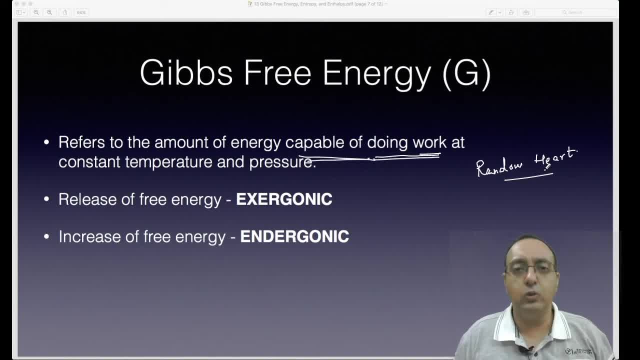 not able to do any work. This is not not contributing to any useful work, But the amount of energy that can be used to do useful work is referred to as Gibbs free energy. it is captured in the form of ATP, So ATP, basically, is the source of free energy for us. 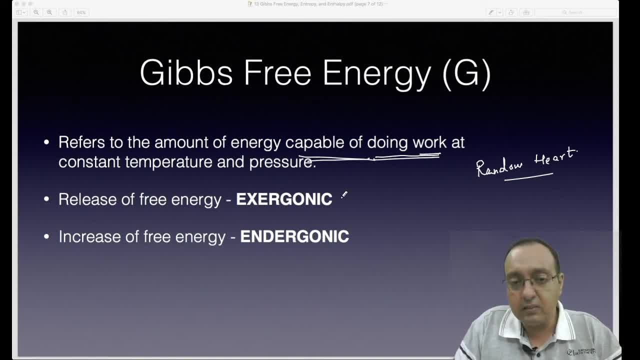 Then a reaction has a release of free energy. This is called an exergonic reaction. So, for example, all the catabolic reactions or most of the catabolic reactions, they are exergonic reactions And reactions which lead to increase in free energy, where we put energy from the 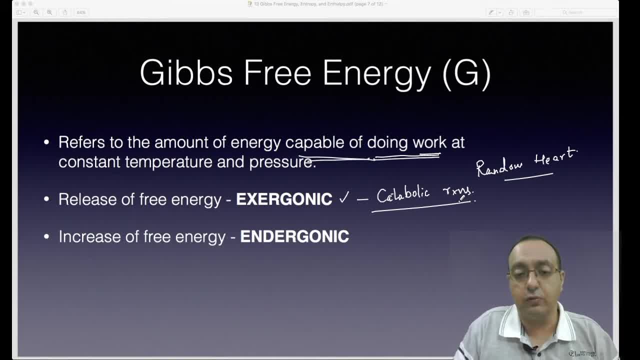 surroundings into the system. those are all endergonic reactions. So, for example, anabolic reactions, synthesis of DNA, synthesis of RNA, star synthesis, cellulose synthesis, all of those things. So this is the concept of Gibbs: free energy. 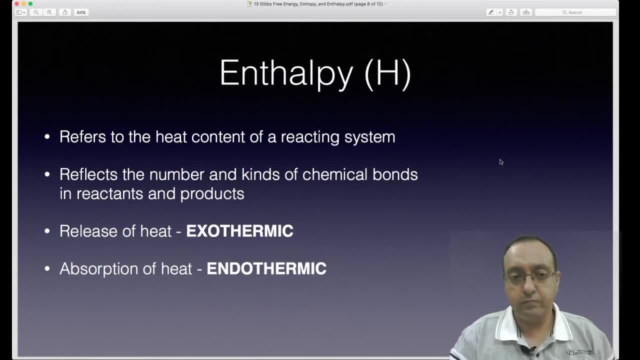 and exergonic and endergonic reactions. The other concept is enthalpy. Enthalpy is denoted by letter H and refers to the heat content of a reacting system. Now it sounds a little bit: what weird is the heat content of a system? but basically it means what is the total bond. 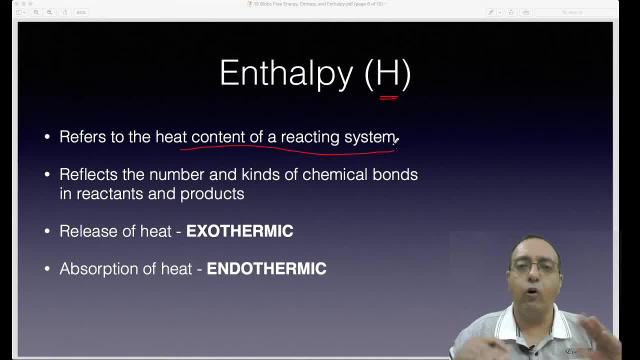 energy of a system, The total- some total- of all the bonds and their bond energies present in the system is referred to as enthalpy. So if, during a reaction, there is production of molecules which have less bond energy as compared to the 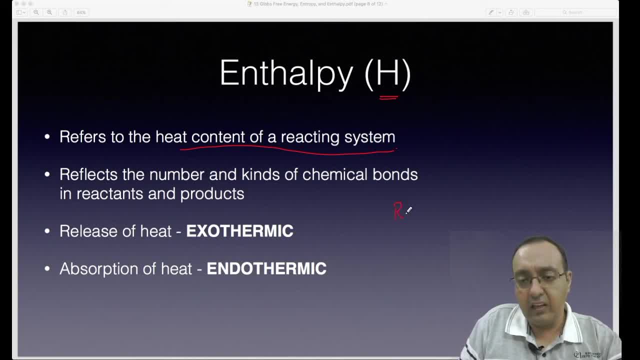 starting materials, reactants. So if there is a reaction where we have the, They lose heat and lead to products. This is called an exothermic reaction- For example, burning of a firecracker- An endothermic reaction. on the opposite, it takes up heat from the system. 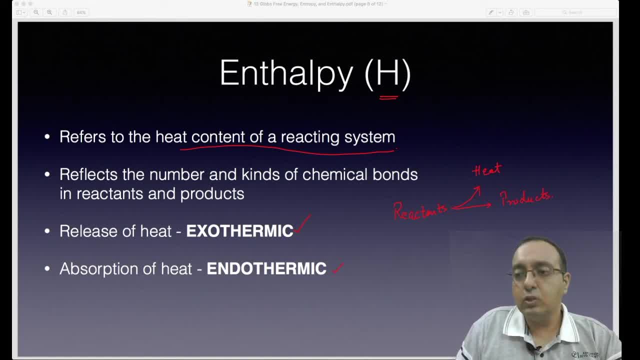 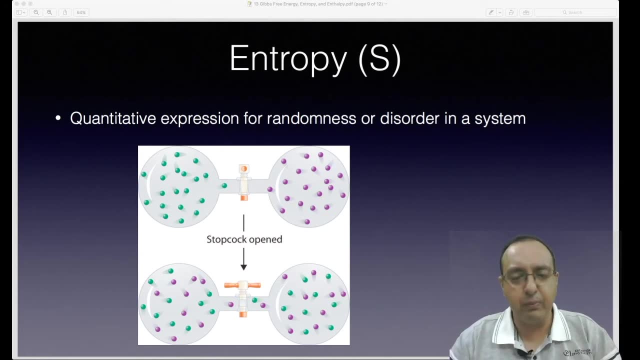 For example, boiling water. So these are concepts associated with enthalpy, exothermic and endothermic reactions, And the last but not the least is entropy, a hugely misunderstood concept, but it's pretty easy to understand. It basically refers to amount of randomness or disorder in a system. 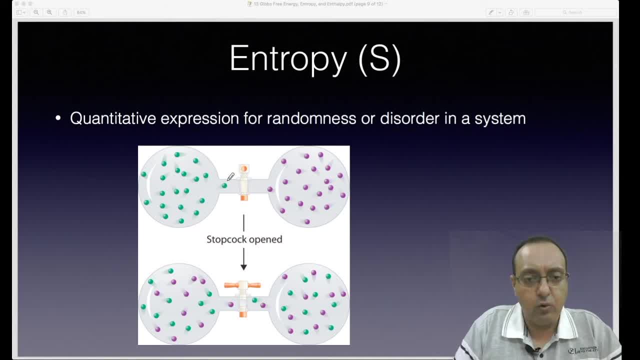 So, for example, here I have an illustration- here You have two glass flasks and these are separated by a stopcock And these have two different gases. Let's say this is nitrogen and this is carbon dioxide, or could be any one. And what happens if we open the stopcock? 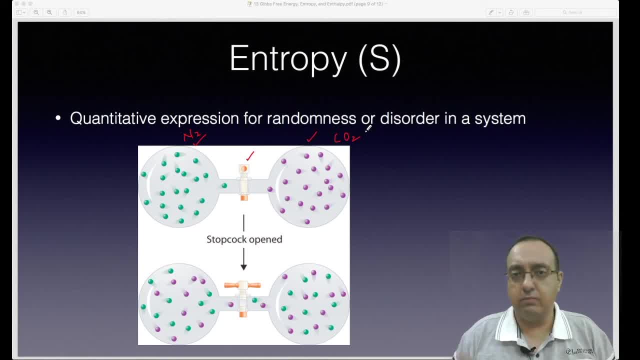 What will happen is due to the random collisions and the random chance. what will happen is, after some time there will be equal, equal molecules in both, the almost equal molecules in both the flasks. That's what the kind of the colloquial meaning is. 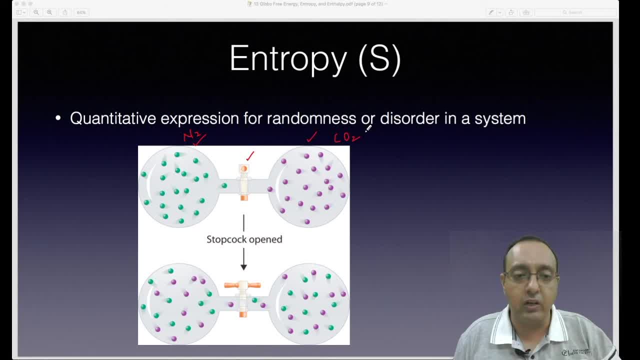 It refers to the amount of disorder in the system. So here they were pretty ordered, And as soon as you open the stopcock, it lent led to this disordered system. So universe tends to, or universe, or all spontaneous reactions lead to increase in entropy. 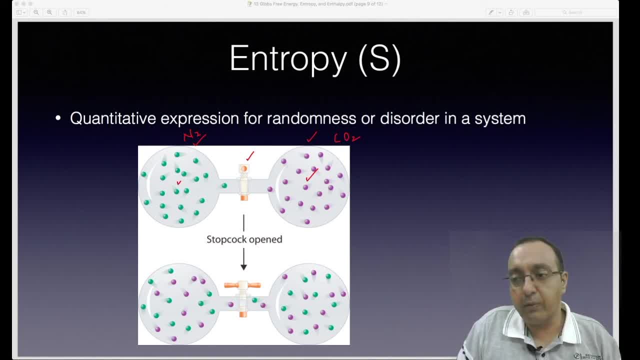 That's what the overall formulation is, although it is a pretty deep topic and you can explore physical chemistry textbooks, for example by Peter Atkins- But I think this is sufficient For us to understand that most of the reactions in biochemistry, as well as any reaction in 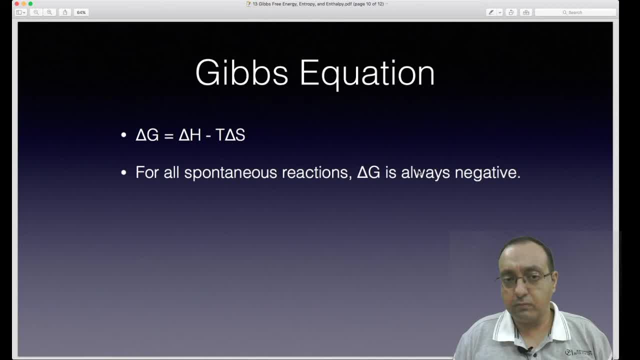 biology involves increase in entropy. And this leads us to our main concept, which is Gibbs equation, which is formulated as: delta G equals delta H minus T, delta S, So this is delta G, which is free energy change. So the delta here refers to the change. 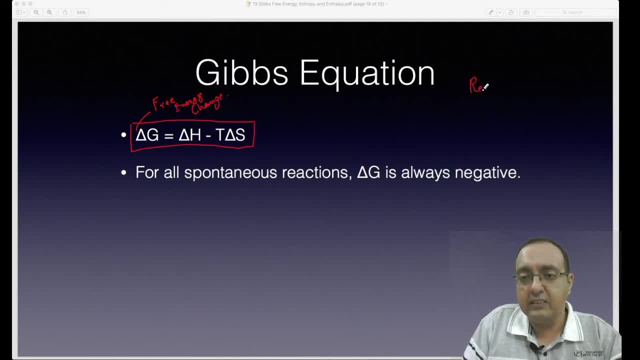 So when we have reactants going to products, what is the change in free energy? So G of R, a standard free energy of reactants and standard free energy of products. So delta G will be Gp minus Gr. Okay, Okay. 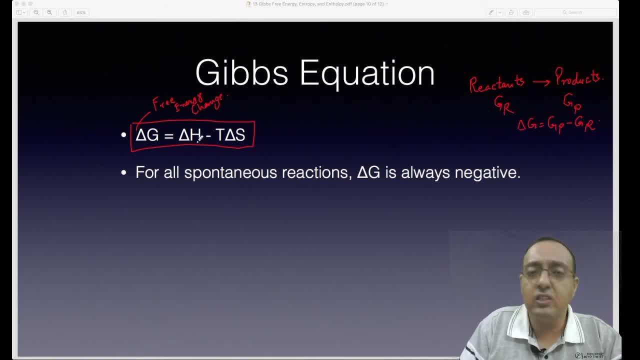 Okay, So that's the change in entropy. Similarly, delta H is the change in enthalpy, T is absolute temperature in Kelvin And delta S is change in entropy. Now, this is the important point here. For all spontaneous reactions, delta G is always always negative. 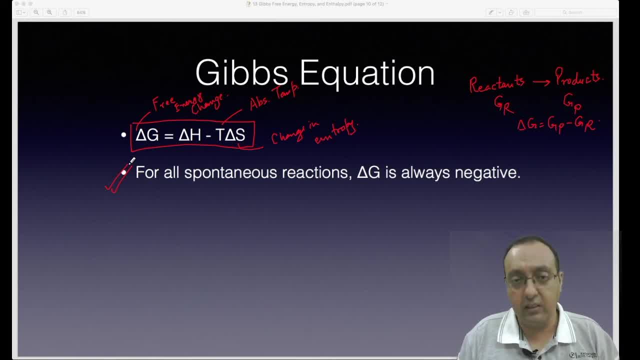 Okay, It has to be negative Okay. This does not mean that you cannot have non-spontaneous reactions happen. You can have non-spontaneous reactions, but you have to provide energy. and that's what organisms do. They provide energy in the form of ATP and ADPH to drive these non-spontaneous reactions, which? 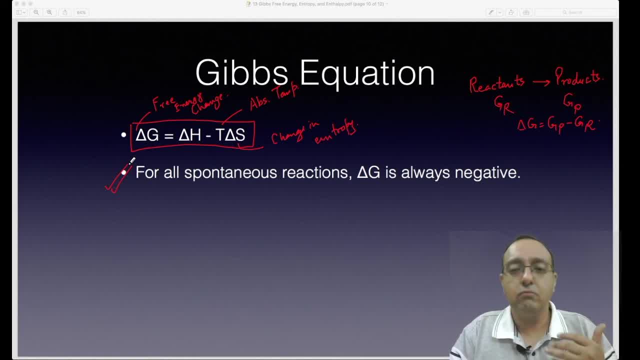 actually decrease entropy. And it is important to note here that Gibbs equation only tells us about the thermodynamics of the system whether a reaction is spontaneous or not. So if the total Delta G comes up to be negative, we say it is a spontaneous reaction. And if total Delta G 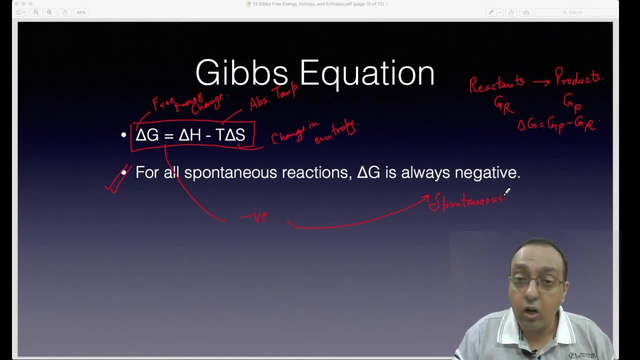 comes up to be positive. we say it is a non-spontaneous reaction, but that does not mean that the reaction will occur very fast. It only says it is possible. For example, you can say glucose- right, You can have a box of glucose, it is present in the air, you can. 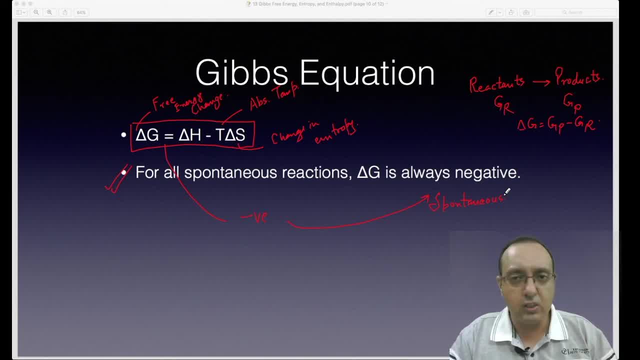 kill it and you can accept glucose or anything of those three reactions as a Sprit Намış without it in your room. oxygen is around it. the oxidation of glucose is a pretty spontaneous process is delta g is highly negative, right? it's somewhere like minus 2840 kilojoules per mole. 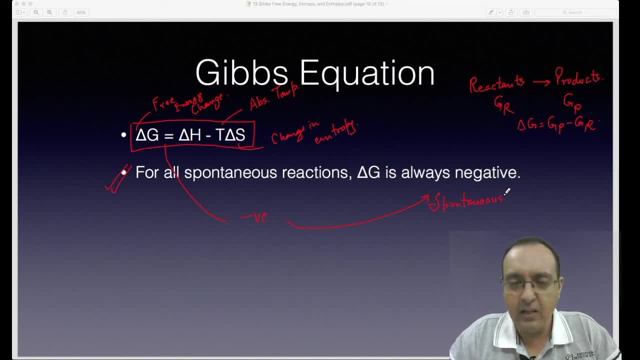 but you don't see glucose disappearing and being oxidized because it does not tell about. tell us about this speed of the reaction, which is the subject of chemical kinetics, not thermodynamics. we are only talking about thermodynamics here. okay, very, very key distinction here. now let's look at some circumstances where we have different. 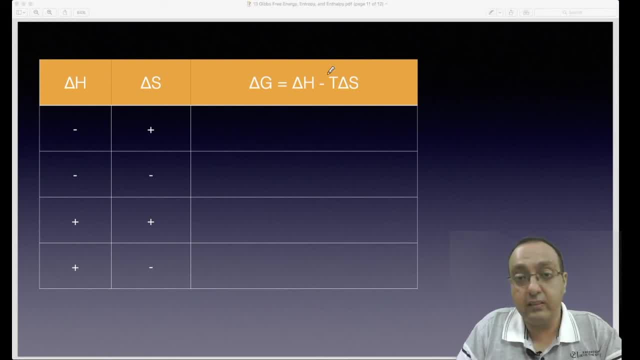 formulations of delta h and delta s and how the how that affects delta g. for example, if in a reaction delta h is negative, that means it is an exothermic reaction and delta s is positive, so entropy is increasing. so this is thermodynamically favored as well as entropically favored. 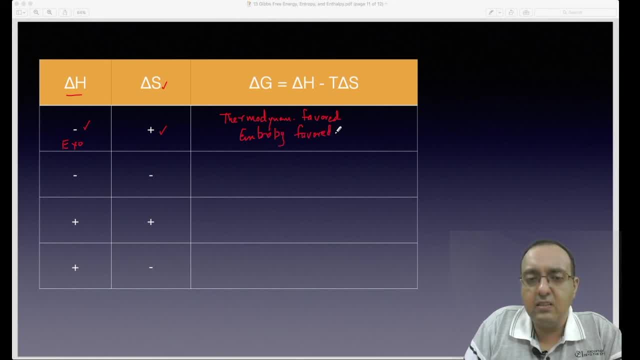 so we can say: this is: this reaction is spontaneous at almost all temperatures. okay, so this is the classical spontaneous reaction. now here we have delta h, which is negative. okay, so that means it is an exothermic reaction. but delta s is negative. that means entropy is. 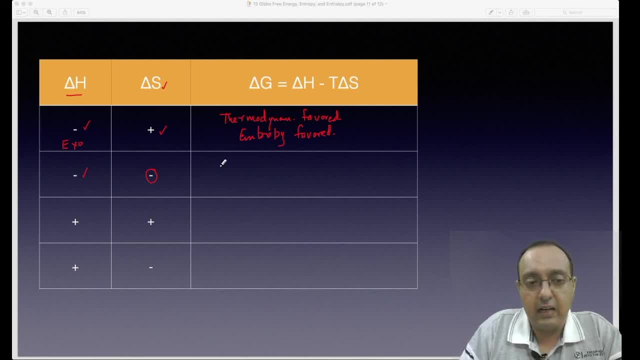 decreasing. okay now, this means that it is not a spontaneous reaction, and it will be spontaneous only when the t will be equal to delta h upon delta s, only at those temperatures, because by the way of entropy it is non-favored, but by the way of enthalpy it is favored. 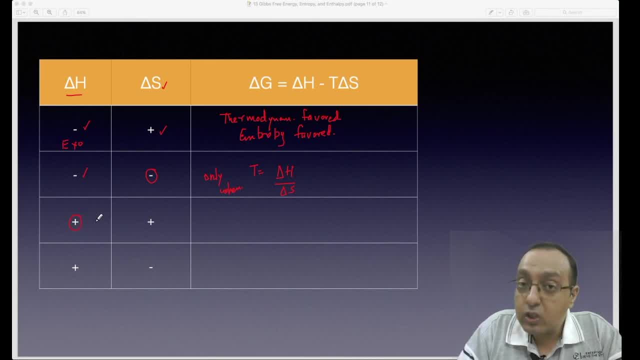 now, delta h here is positive, which means it is an endothermic reaction, and delta s is also positive, which means it is leading to increase in entropy. so this is also a similar situation. so it will only be spontaneous when t equals delta h upon delta s and, last but not the least, where delta h is positive.